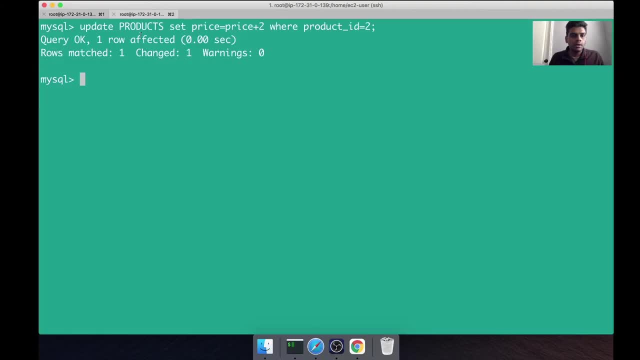 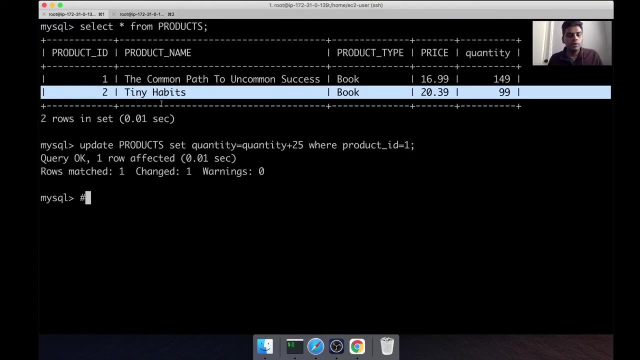 this grow and this guy is holding a roll level. knock on this roll. So this was fine, Right, So we are operating on different records, two different locks, independent of each other, all good. so now let's say, on the same seller, the second person who is updating the price. 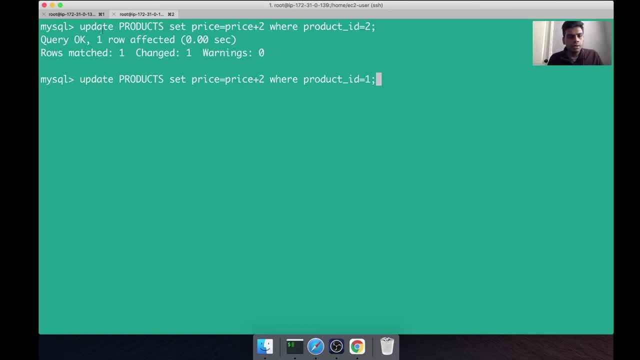 wants to update the price of this other book to actually like he is actually increasing the price again by two dollars. of this book, the product ID equals one. which book this one right here. let's go ahead and try to increment the price by running this command. you know he's waiting on waiting. 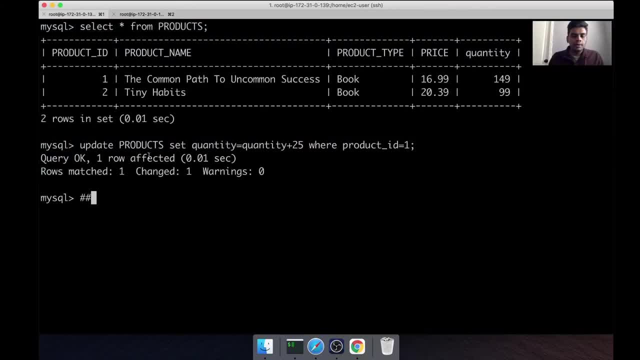 for the lock, actually exclusive lock- and that's not available because this seller has not committed, actually it is not committed. so let's actually go back here and and this seller at the same time tries to update the price of the other book, which book actually has two dollars of this book? 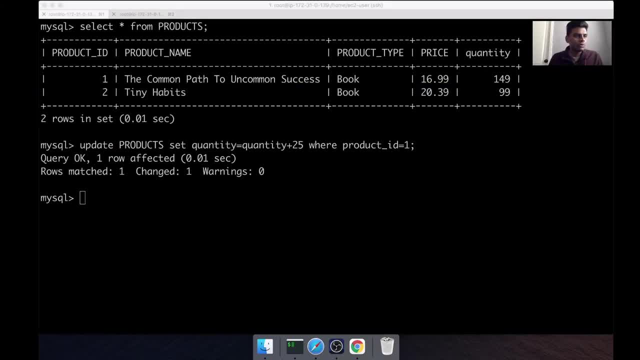 the price of or quantity of this book. so two sessions are fighting for pretty much the same resource. you know, we ended up in a deadlock situation, so my sequel was smart enough to just kill the session, otherwise we would have two sessions waiting for each other endlessly right. so here you can see the 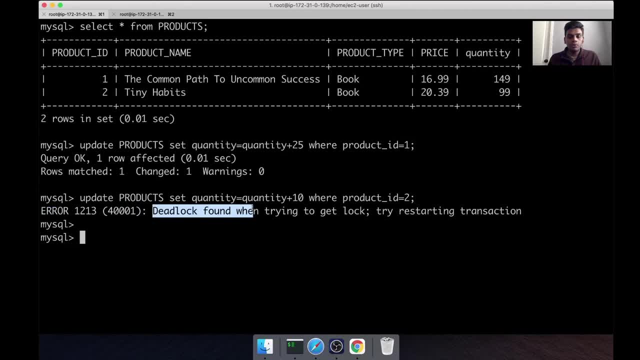 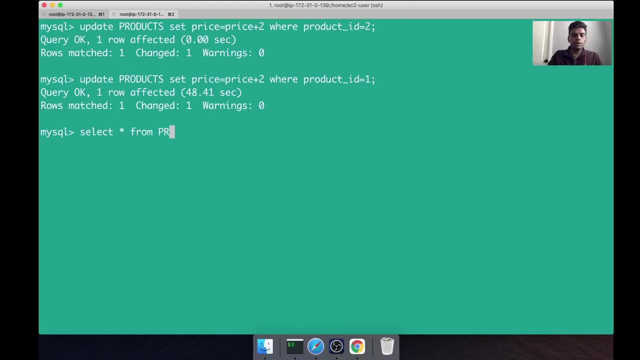 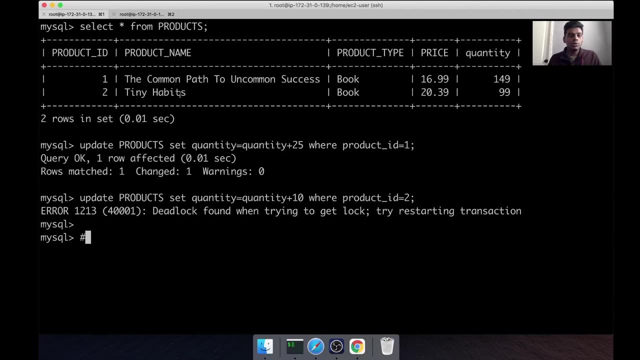 error code that is thrown. it says deadlock found when trying to get lock and try restarting the transaction. so let's go ahead and query the products table and see how it looks. you can see that this whole transaction was rolled back correct, with both the transactions were rolled back. this, even this one, was. 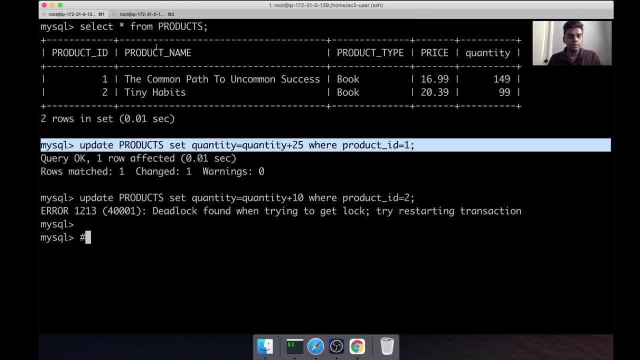 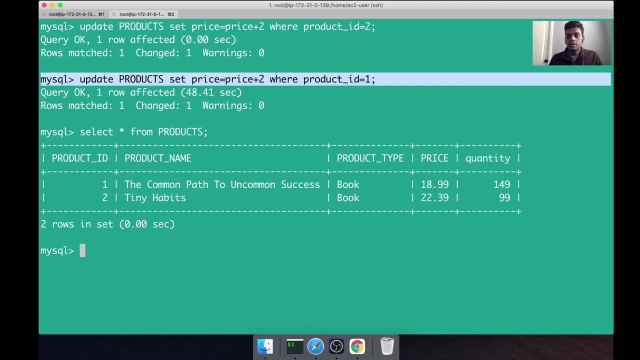 rolled back, so I think that lock was also killed. that's why this is deadlocked. this one went through and, if you can see, the prices have increased by two dollars, like because initially it was 1699 and 2039 and here 1899 and 2239. okay,